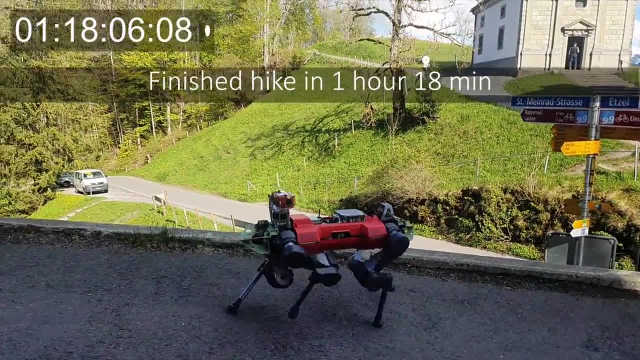 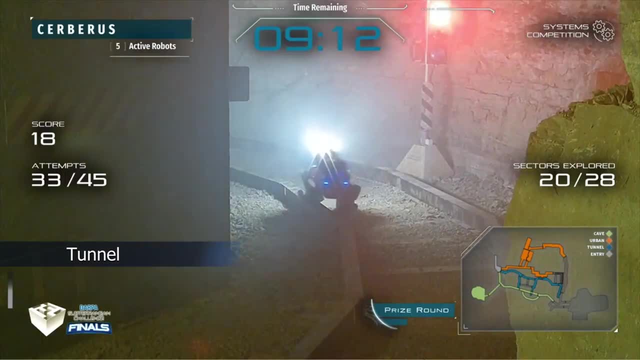 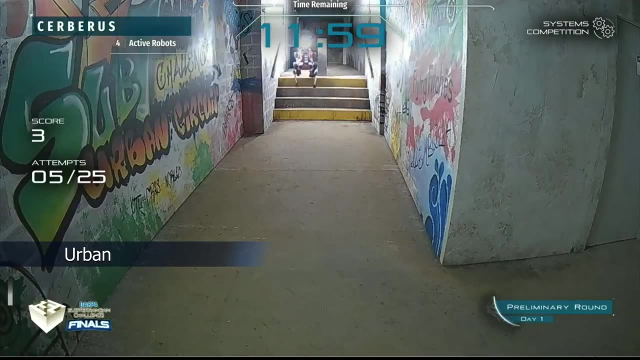 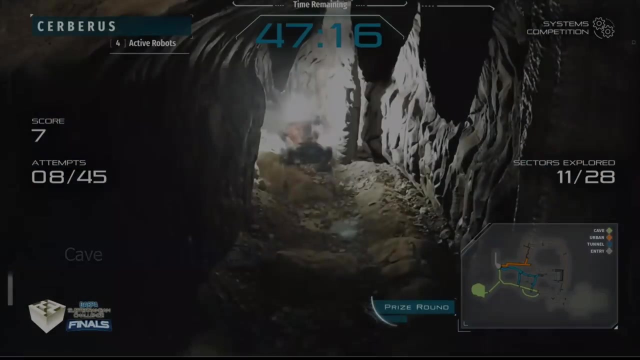 Despite all the challenges, the robot finished the hike without any human help and without a single fall. It completed the hike in virtually the same time as suggested by a hiking planner. The robot also enabled autonomous operation in the DARPA subterranean challenge, where Team Cerberus deployed our locomotion controller autonomously over extended periods of time in underground environments with rough terrain and degraded sensing. 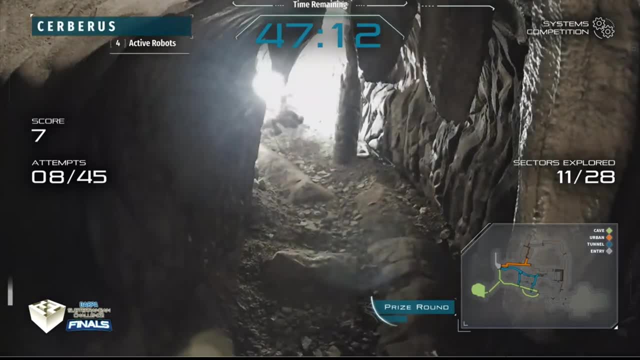 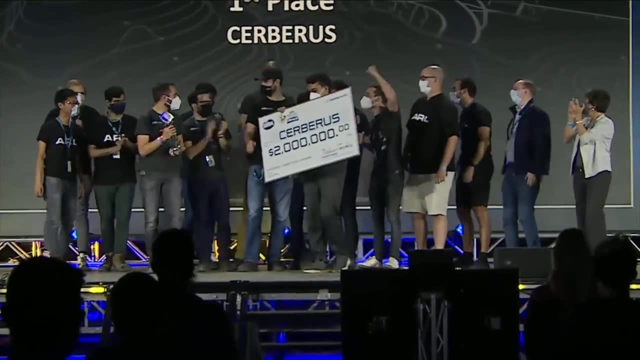 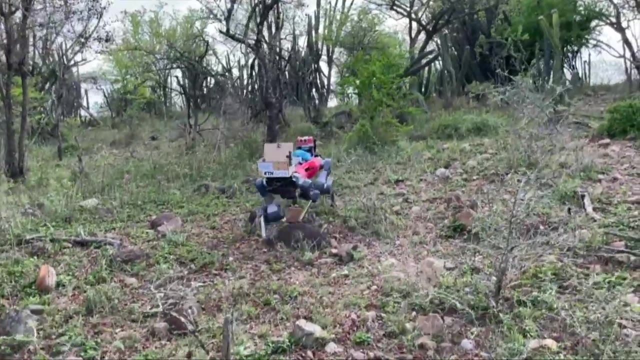 Our locomotion controller explored the underground environments over 1.7 kilometers per day. Toouts of about 1.1 meters were occupied 1.7 kilometers without a single fall, helping Team Cerberus win the first prize. Our controller was also used in South Africa, traversing natural environments. It enabled research on the interaction between robots and animals. 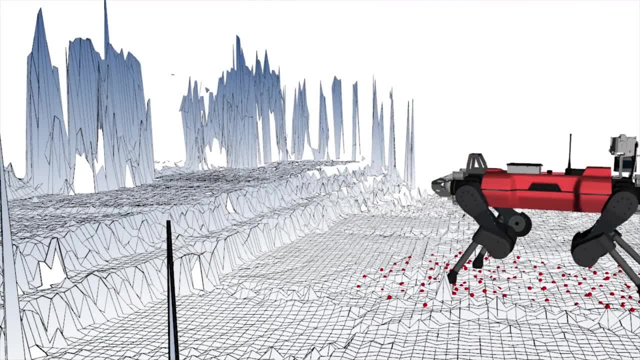 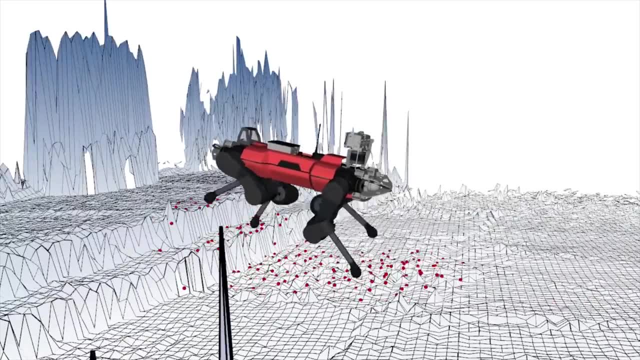 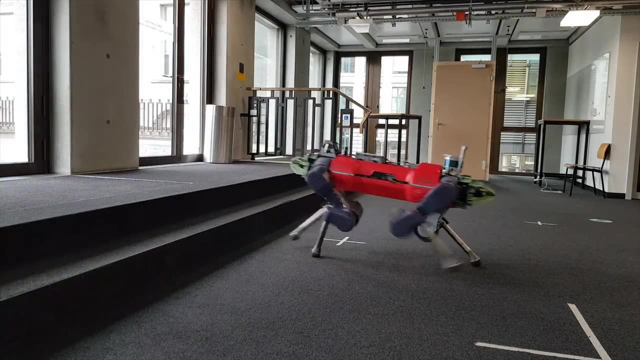 Here is how it works: The robot builds a local height map and samples the relative terrain height around each foot. The locomotion controller utilizes this information to anticipate upcoming terrain and perform smooth locomotion over obstacles. However, this map information frequently becomes unreliable in the real world. 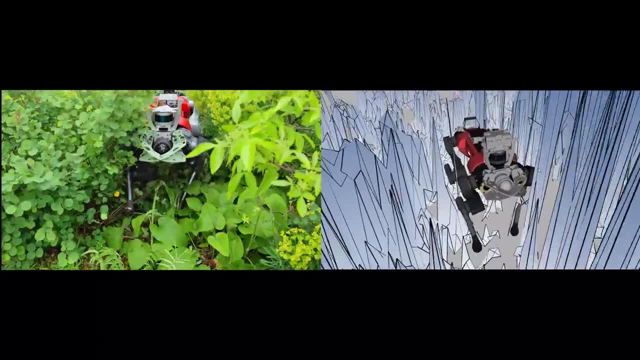 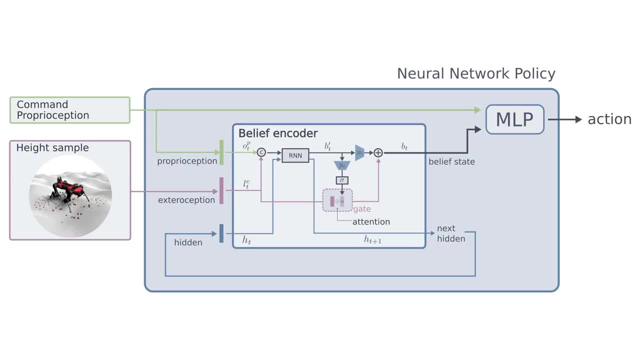 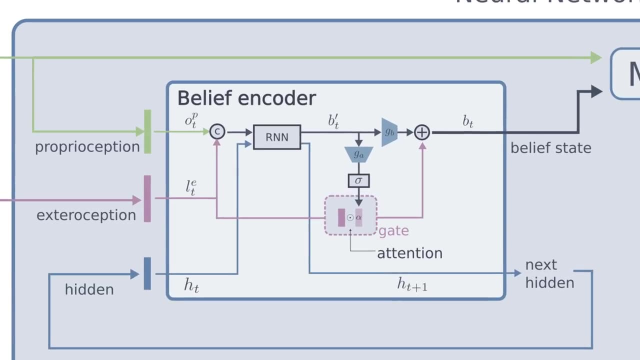 To remain robust under such conditions, the controller has to learn to ignore misleading exteroception and rely on proprioception. instead, We introduce an attention-based recurrent encoder that combines proprioception and exteroception into an integrated belief state. We employ an attention mechanism that allows direct access to exteroception when it is reliable. 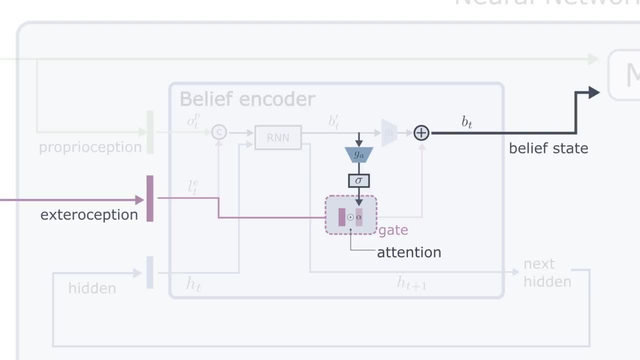 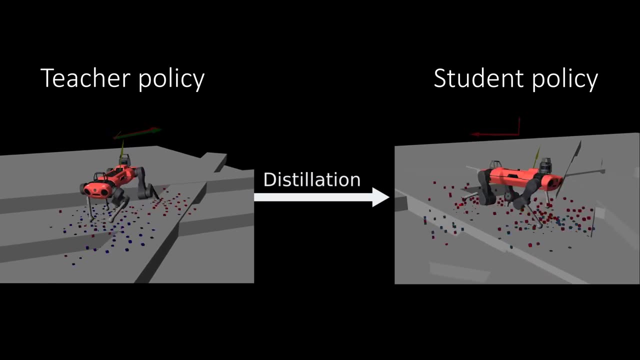 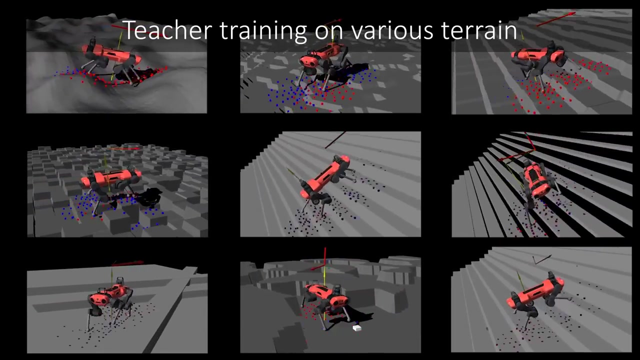 but learns to discount it when exteroception is degraded. We employ a privileged training procedure. We first train a teacher policy on a variety of terrain using reinforcement learning. The teacher policy has privileged access to all ground truth information from the simulator and learns an optimal. 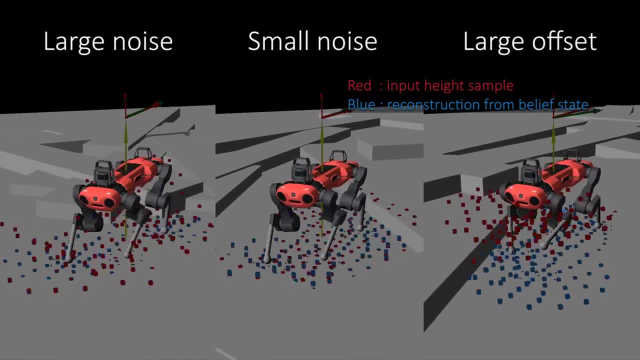 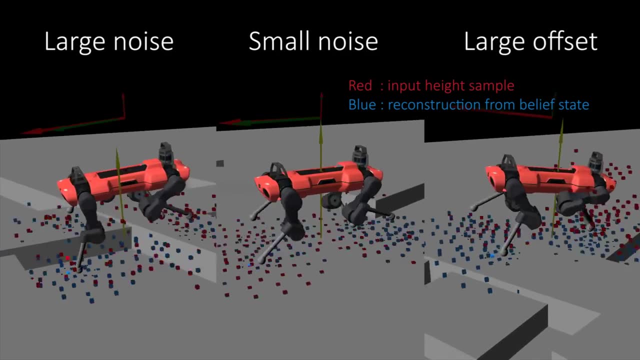 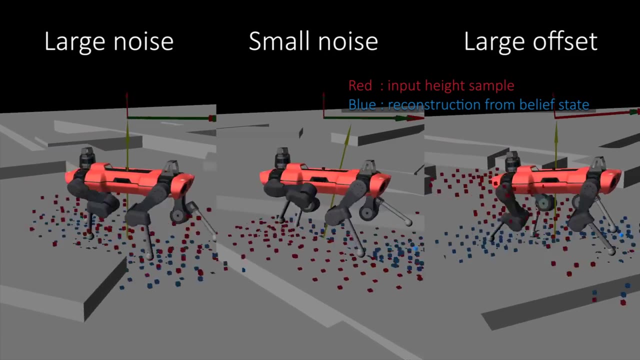 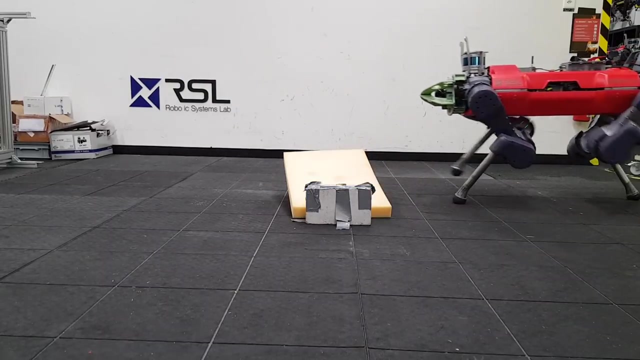 reference motion. We then train a student policy to imitate the teacher policy. given observations of varying reliability, The student contains the belief encoder and also tries to reconstruct the ground truth height samples to encourage an informative belief state. This is illustrated in this controlled experiment where the robot walks over a soft foam block which appears solid but cannot support a foothold. 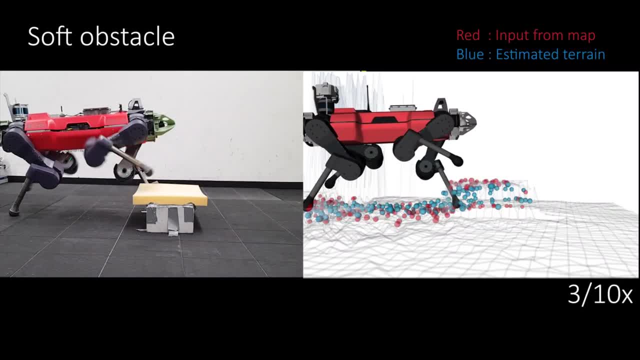 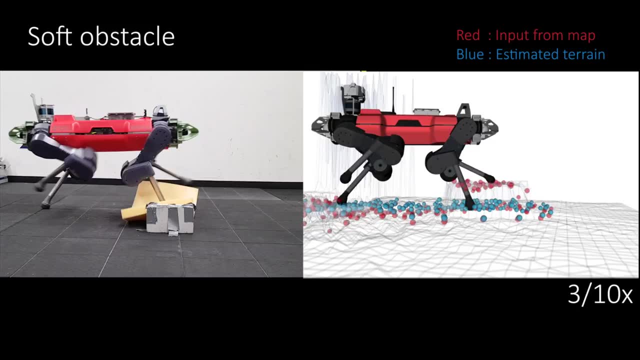 When the robot tries to step on the compliant surface, the sinking foot contradicts the anticipated terrain profile and the policy immediately revises its internal belief about the terrain. This estimate remains intact as the robot continues stepping due to the recurrent structure of the encoder.